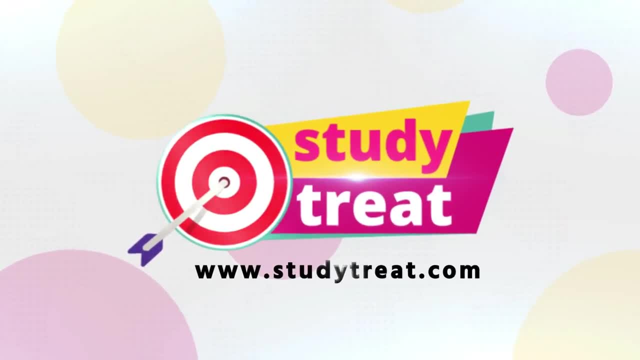 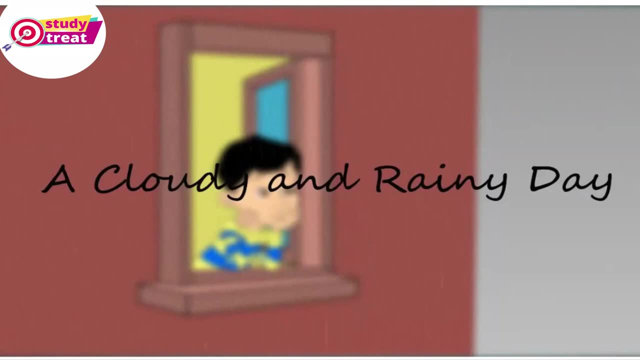 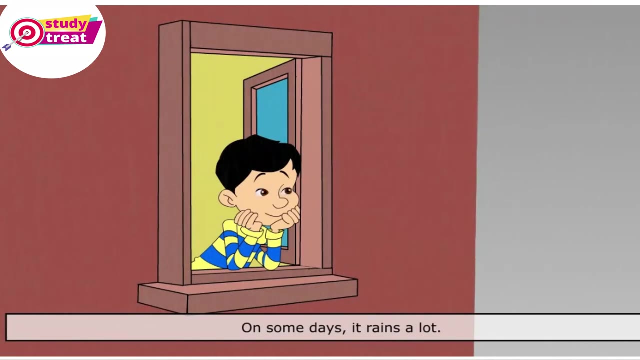 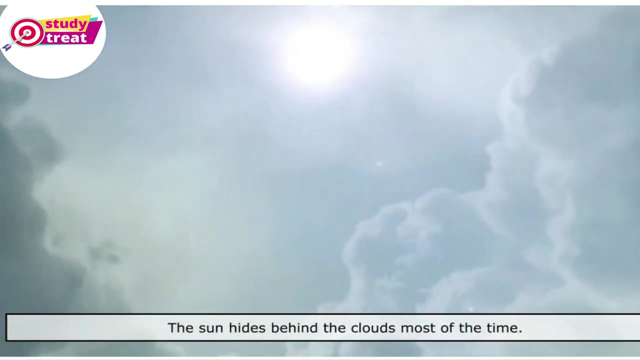 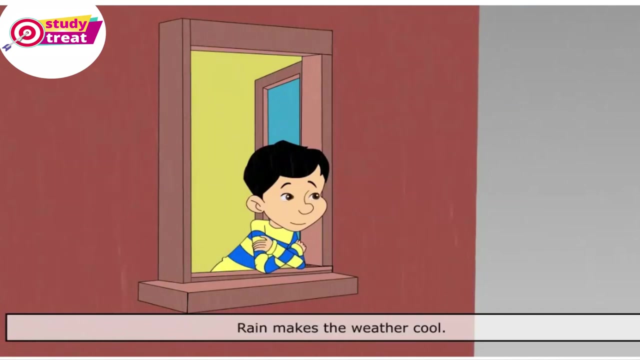 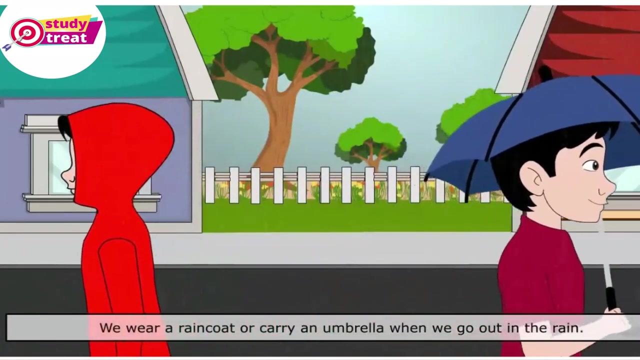 A cloudy and rainy day. On some days it rains a lot. The sky is covered with clouds. The sun hides behind the clouds. most of the time, Rain makes the weather cool. We wear a raincoat or carry an umbrella when we go out in the rain. 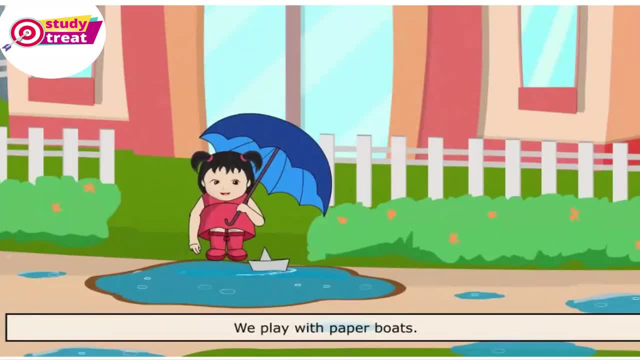 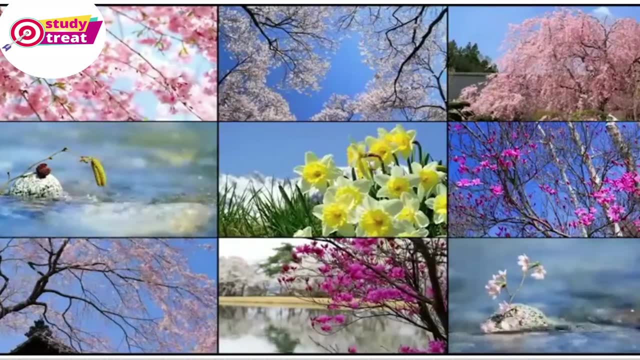 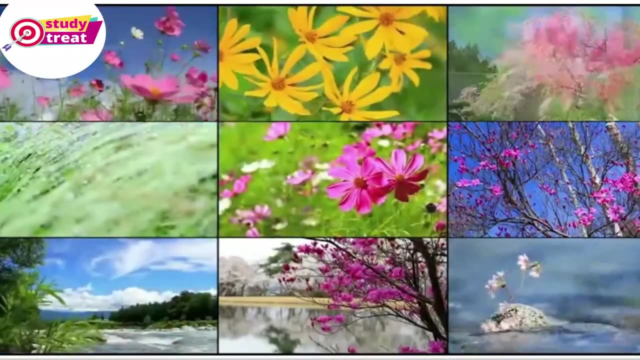 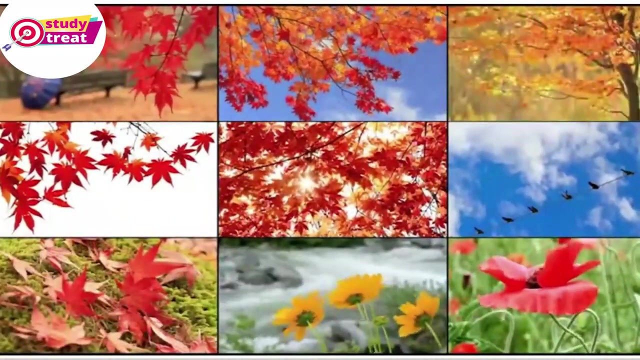 We play with paper boats. Sometimes we see a rainbow in the sky after the rain. We have four seasons in India. They are spring, summer, autumn and winter. Flowers bloom in spring. We can see many birds Also around. Summer is very hot season and the sun shines brightly in the sky. 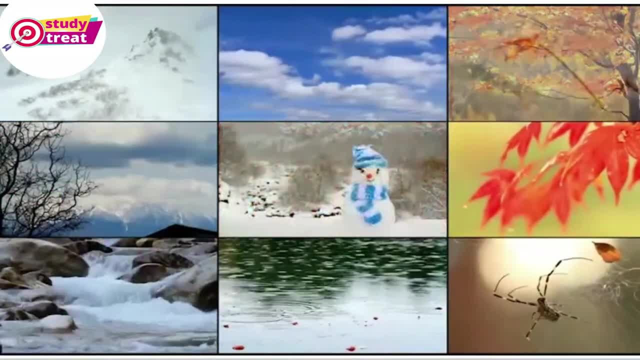 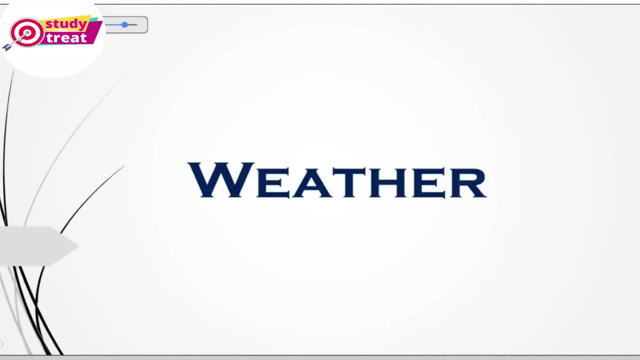 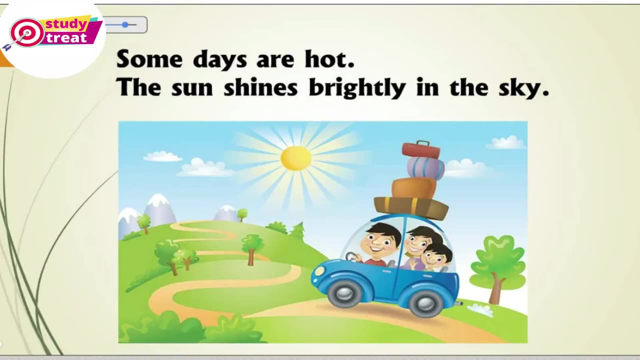 In autumn many plants shed their leaves. Winter is the coldest season. On some mountains, snow falls. We like to make a snowman with snow Weather. Some days are hot, The sun shines brightly in the sky. We wear cotton clothes to stay cool. 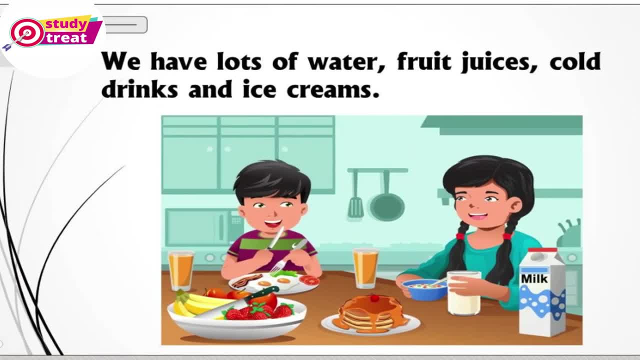 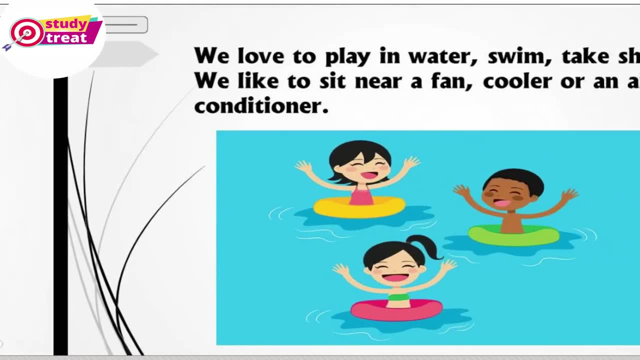 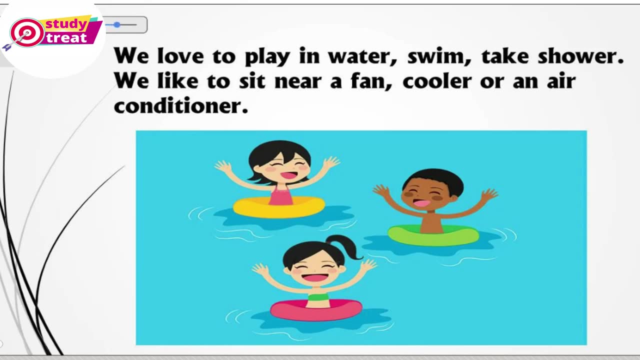 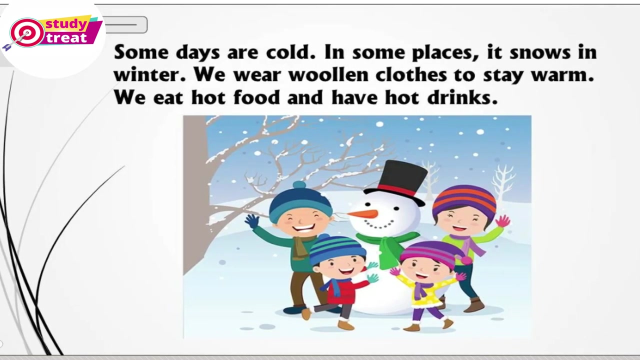 We have lots of water, fruit juices, cold drinks and ice-creams. We love to play in water, swim, take shower. We like to sit near a fan, cooler or an air conditioner. Some days are cold. In some places it snows in winter. 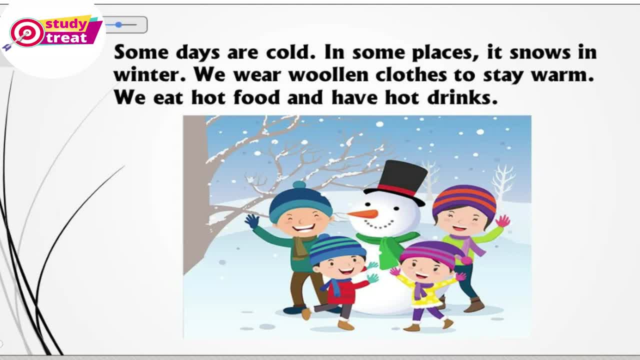 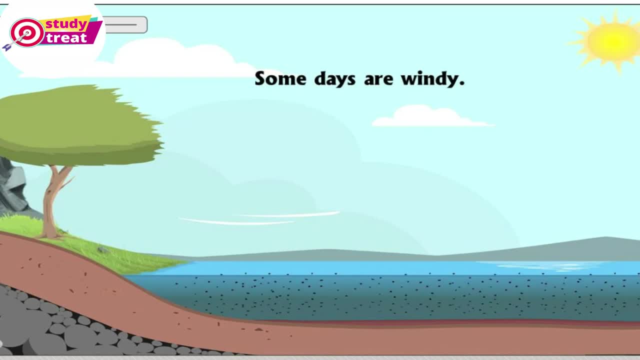 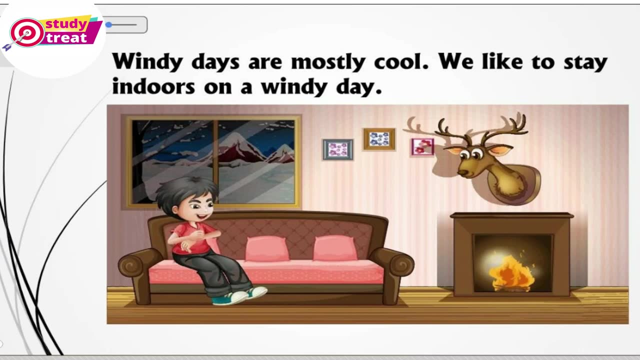 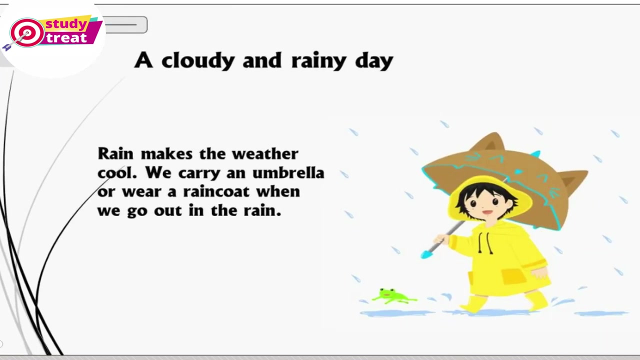 We wear woolen clothes. We wear woolen clothes to stay warm. We eat hot food and have hot drinks. Some days are windy. Windy days are mostly cool. We like to stay indoors on a windy day, A cloudy and rainy day. 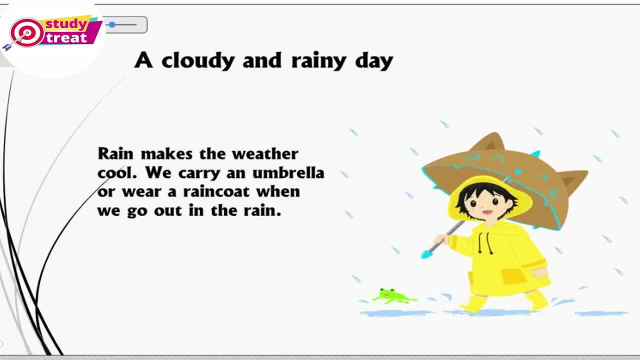 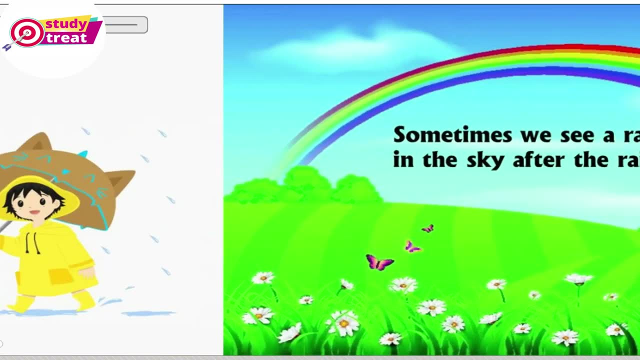 Rain makes the weather cool. We carry an umbrella. We carry an umbrella or wear a raincoat when we go out in the rain. Sometimes we see a rainbow in the sky after the rain.